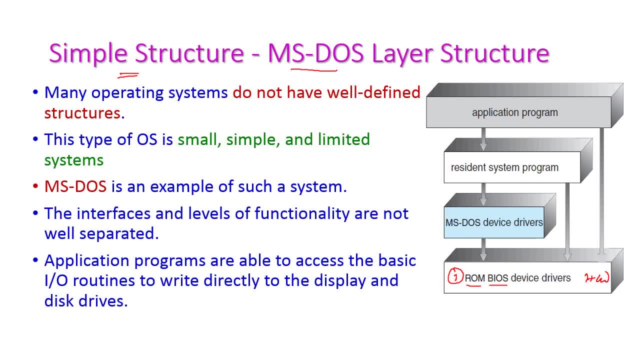 read-only memory BIOS. basic input and output systems and other device drivers are there, and this is the second layer. this is OS layer, which OS? MS-DOS OS- okay, and this is the third layer. we are having system program And this is the last layer, application program. okay, Hence this structure is very small, simple. 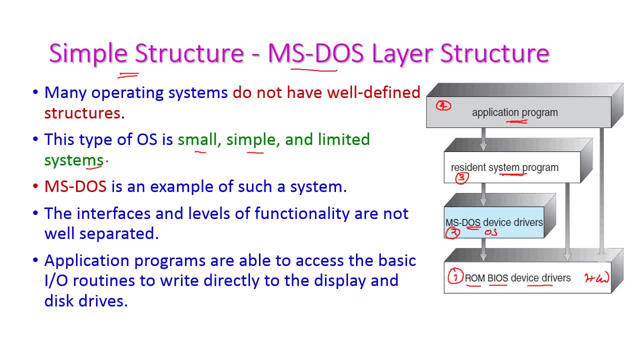 so it is having very limited functionalities. okay, and in this structure the interfaces and levels of functionalities are not well separated. That means the system programs and application programs can also directly access the hardware. okay, system programs and application programs can also directly access the hardware, okay. 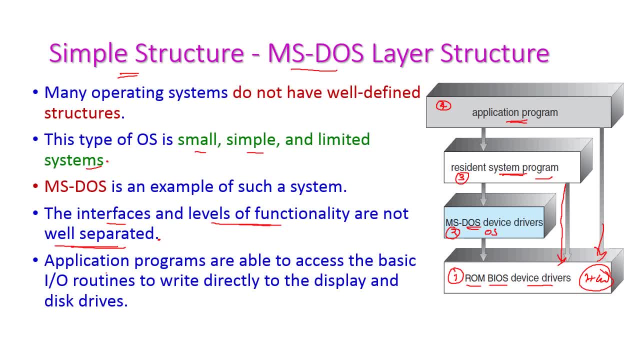 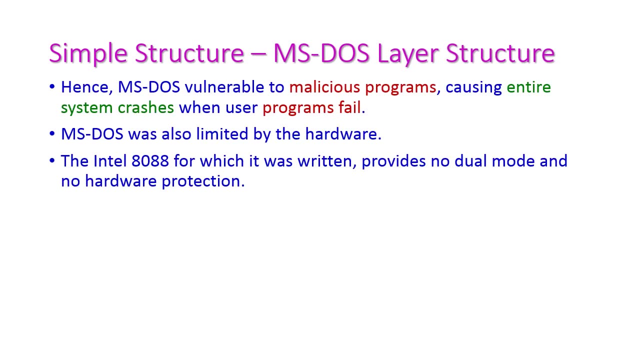 Application programs can also directly access hardware: See application programs are able to access the basic I-O routines to write directly to display and the disk devices, If all the layers can access the hardware directly. hence the MS-DOS will be vulnerable to malicious program. That means all the virus or any other malware program can easily affect or attack this MS-DOS, which causes the entire program crashes when the user program fails. 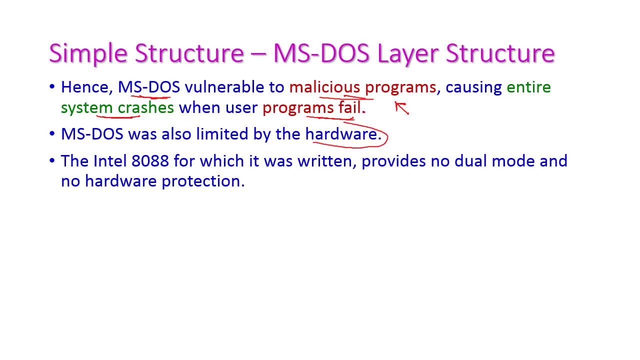 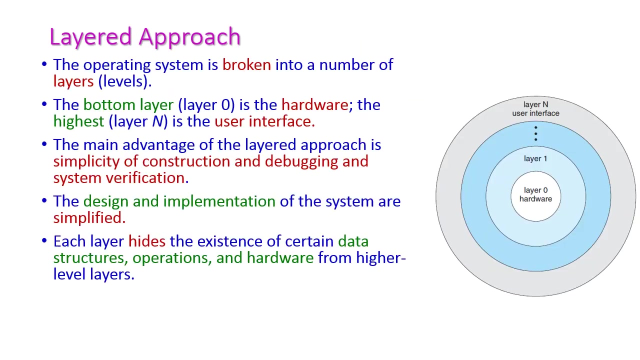 And it is having a limited hardware, also because the MS-DOS is written for the processor 8088, okay, by using the assembly language, and it provides no dual mode and no hardware protection. The second one is layered approach. Here the operating system is broken into number of layers. Layer is otherwise called as levels. 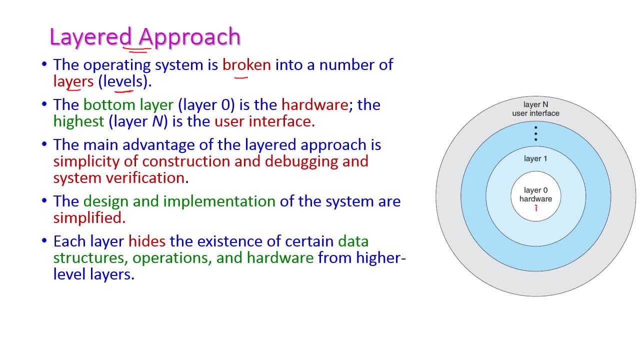 So in this diagram we are having MS-DOS hardware layer. This is layer 0.. And finally we are having user interface layer. In between we are having some other layers also. OS layer may be here. Okay, the bottom layer is hardware layer and the topmost layer is user interface layer. Okay, and the main advantage of layered approach is the simplicity of the structure, and debugging and system verification is very easy. 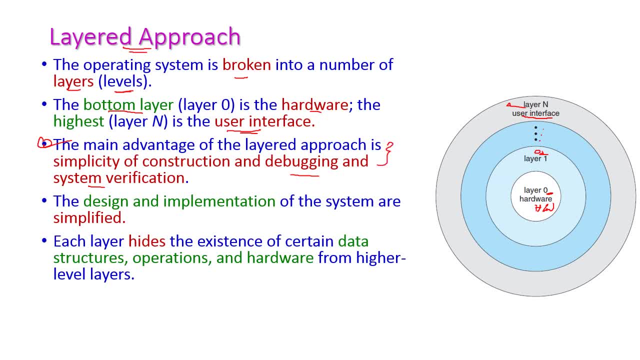 Okay, and the design and implementation of the system are very much simplified when compared to the previous. the simple structure: Each layer hides the existence of certain data structures, operations and the hardware from higher level layers. Okay, here the layer 1 will access layer 0, and the layer 2 will access layer 1, and layer n will. 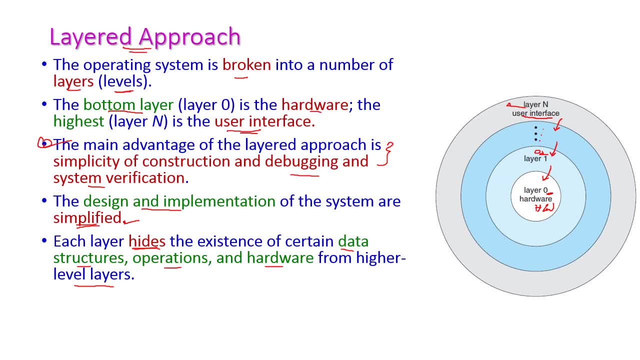 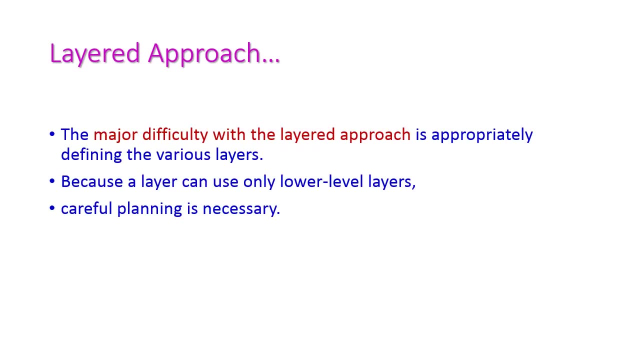 access layer n-1.. So the access will go in this way. Hence, each layer will hide the data structure, operations and hardware from higher level layers. The main difficulty of this layered approach is defining the various layers, How we are going to define each and every layer. 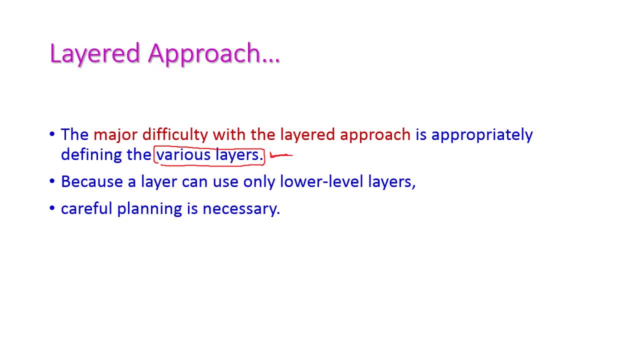 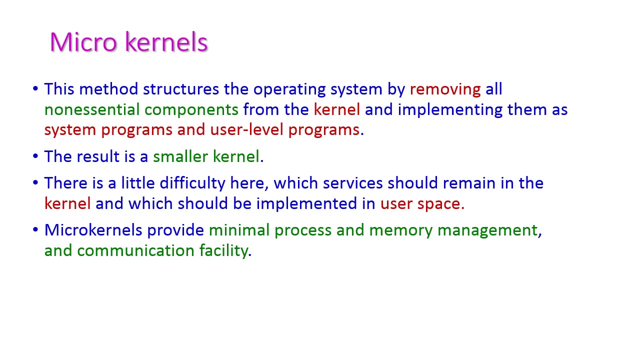 That is, we need to separate the functionalities to the layers, Because the higher level layer will use only the lower level layers. Hence the careful planning is very much necessary here in this layered approach. The third structure is microkernel structure, Means the non-essential components will be removed from the kernel. 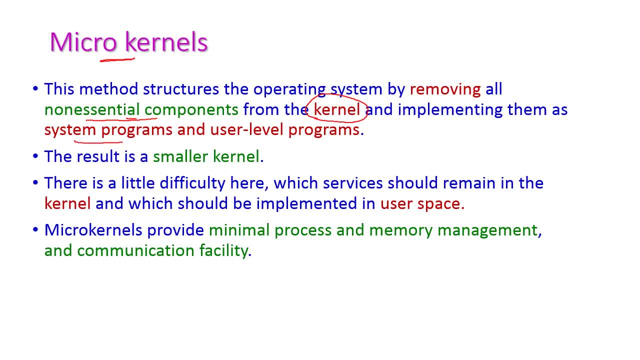 And those will be moved to either system programs or user level programs. Hence the size of kernel will be very much Reduced to, that is, to microkernel. Here we will face very little difficulty, That is, which service should be in the kernel. 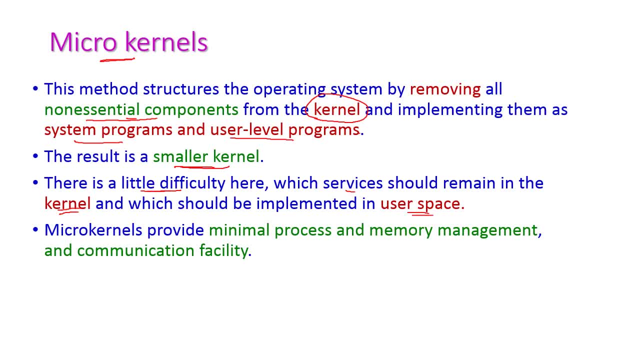 And which service should move to the user space. That means we are going to remove the unessential component from the kernel, Hence we should have some knowledge about which component will be the unnecessary And that will be moved to user space. The microkernel will provide. 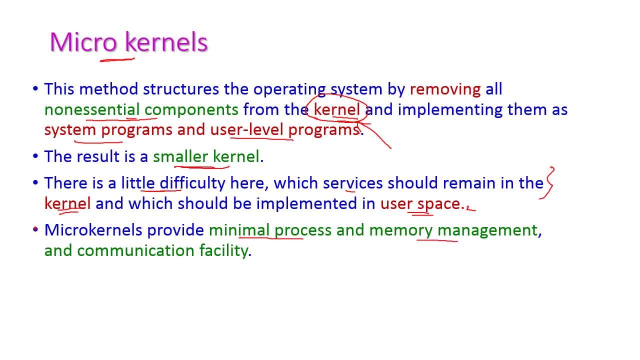 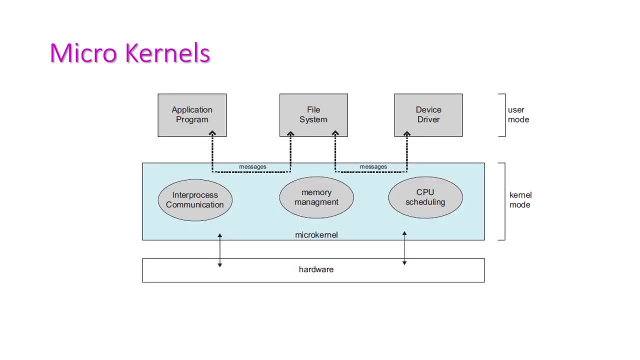 Minimal process memory management and communication facility. And this is the example for microkernel. here, The layer one which is hardware, All the hardware will be there, And this is OS layer. second layer From this OS layer, The inter-process communication, memory management and CPU scheduling will remains in the kernel mode itself. 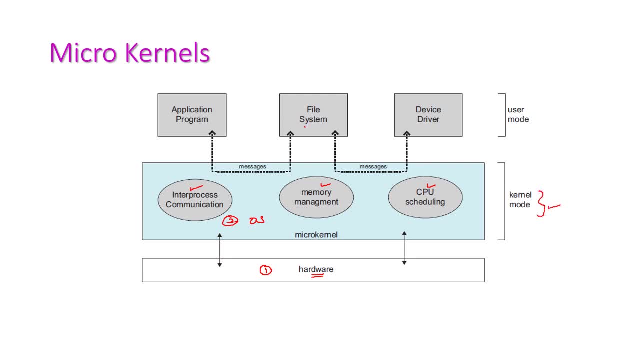 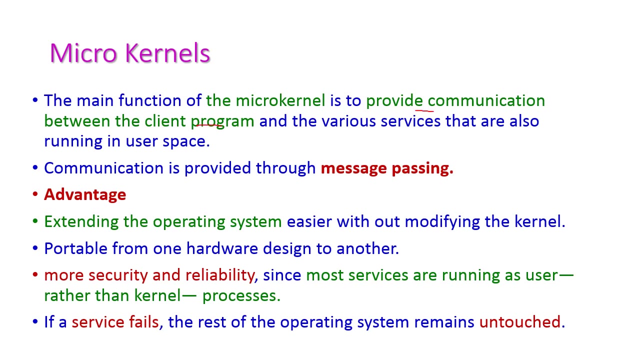 And the CPU scheduling will remains in the kernel mode itself And we can move this file system and device driver to the user mode. Hence the size of kernel will get reduced. The microkernel provides communication between the client program, Because maximum services will be run only in the user space. 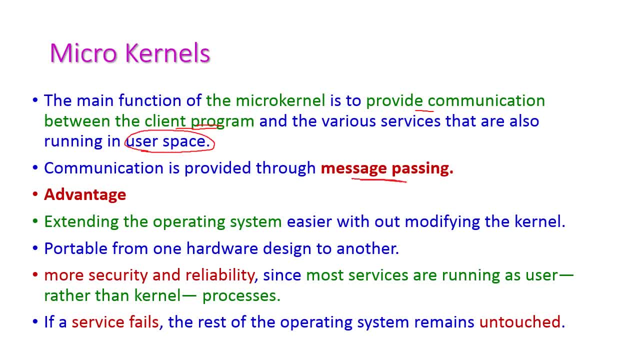 And the communication will be taken place through message passing. And let us see the advantages: Extending the operating system is very easy, very easy, without affecting the kernel or without modifying the kernel. We can easily extend the functionalities. Maximum functionalities will be run in the user space only and portability. 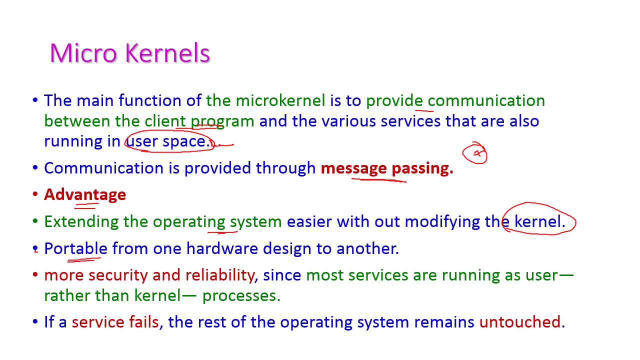 is another advantage. We can easily move the operating system from one hardware to another hardware and it is more security and reliability, since maximum services will run in the user, not the kernel mode. If any of the service fails, then the rest of the operating system remains. 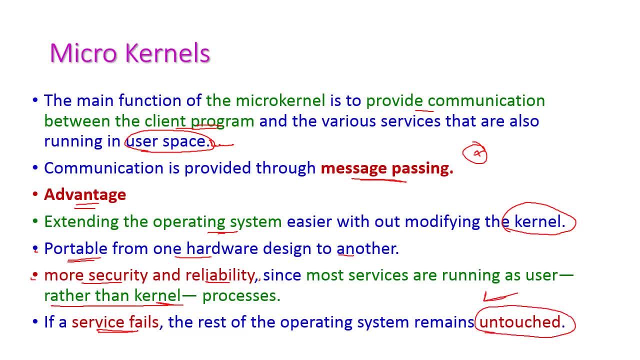 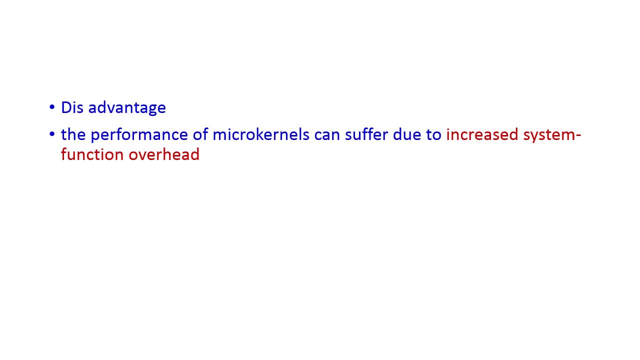 untouched. That will not affect the kernel. The only drawback of microkernel is it will suffer due to increased system function overhead because we cannot decide the function that should be either run in the user mode or in the kernel mode. We need to decide that carefully, otherwise the microkernel structure will get 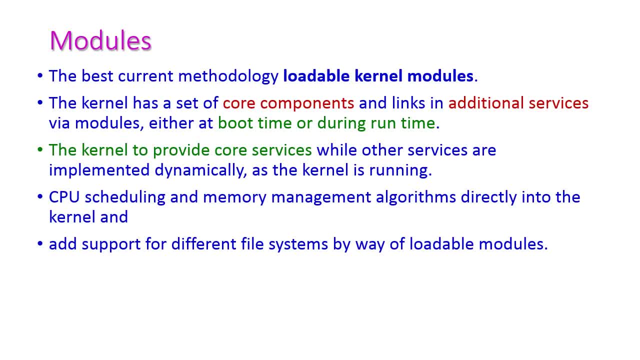 failed. The fourth one is modular structure. The current operating system will follow only these modules, ie loadable kernel modules. Here the kernel has the core components, ie core modules, and it is having links in additional services. We need to make sure that the kernel has the required services by those modules either. 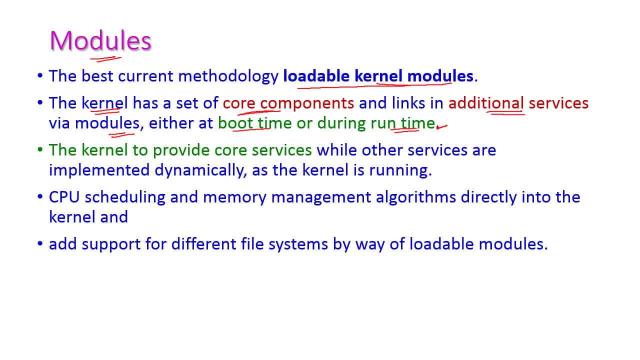 by the boot time or the runtime. So, on demand, the services will be loaded into the kernel and the kernel provides core services. All the core services will be loaded only in the kernel and other services are implemented dynamically. So, based on the requirement,